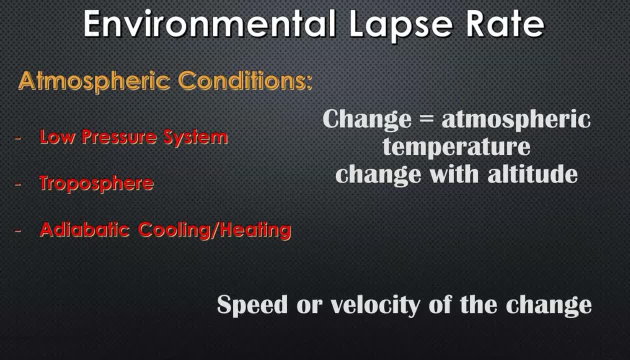 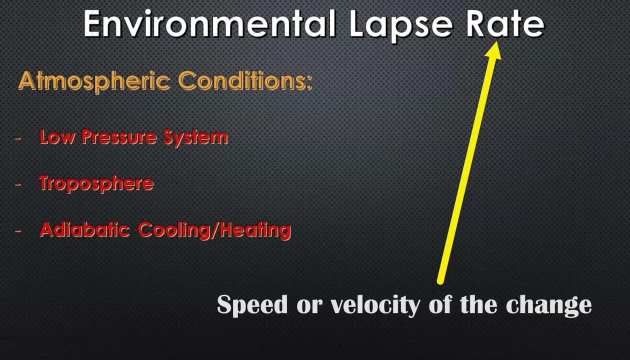 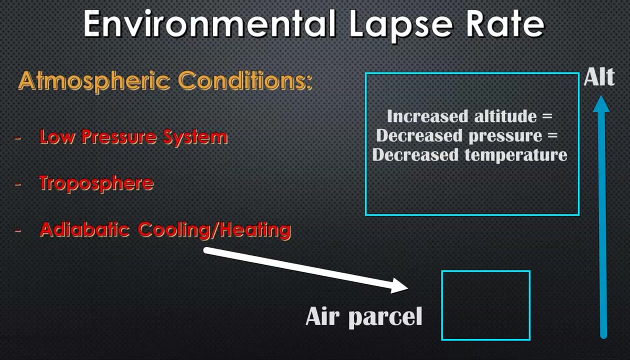 In whatever. in this case it's temperature, and the rate would be the speed or velocity. So how fast does the air change temperature? when we increase in altitudes, we go higher up in the atmosphere And this is the environmental lapse rate. So, looking at the speed at which it cools down, So this is also to do with adiabatic cooling, which is the change of temperature through the difference in pressure, And this change has no additional heat added or taken over. 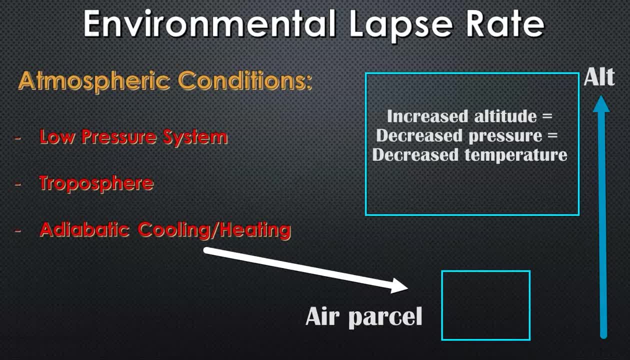 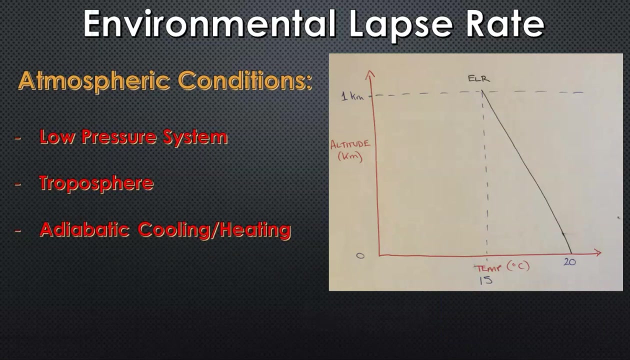 It's just the change of pressure which creates the difference in temperature. So as pressure increases, so does the temperature. as pressure decreases- which is cooling- gets higher, pressure decreases, you will get the air temperature also decreasing. This is called adiabatic cooling. So we discussed the lapse rate. we discussed adiabatic cooling, natural. So if you look at our troposphere- and I've done a graph here on the right hand side, which is looking at an altitude of the surface up to the atmosphere, 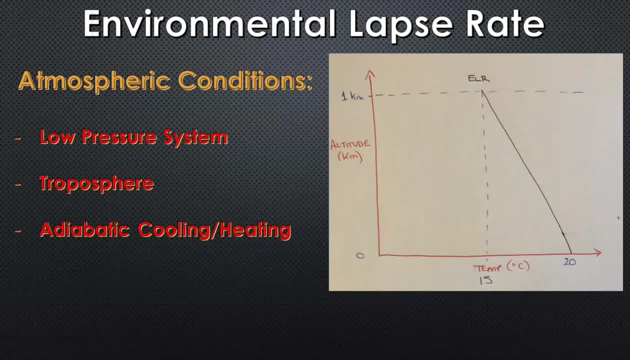 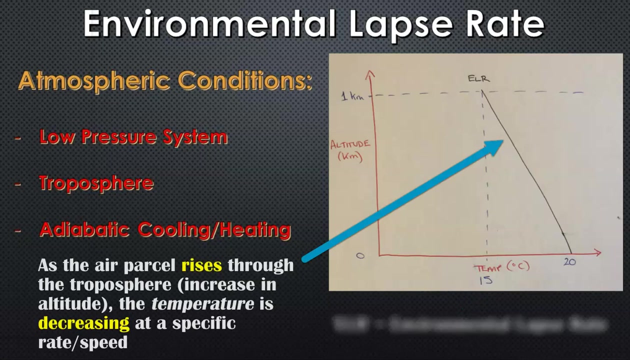 To one kilometer or one kilometer or 1000 meters. Now the ELR is the abbreviation for the lapse rate And I looked at the bottom x axis, which is temperature. So I've put in there that this black line is representing the environmental lapse rate and how it shows that as you increase in altitude the temperature is going to decrease, as shown by the graph. So it starts at 20 at the surface and goes down to 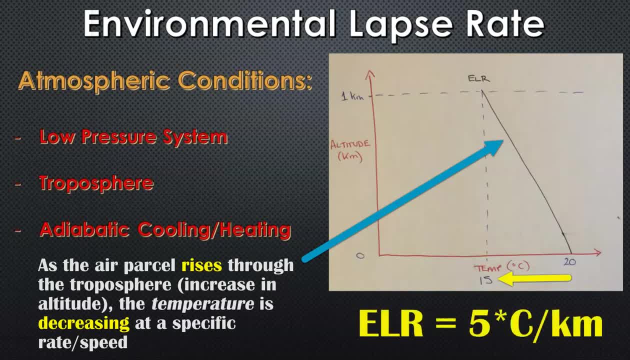 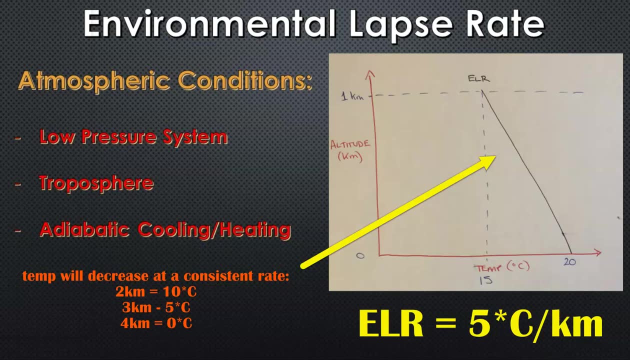 15 degrees Celsius at one kilometer altitude. So it has a lapse rate of five degrees Celsius per kilometer. So we assume that if it stays the same, that two kilometers temperature would be 10 degrees, or three kilometers it will be five degrees. So go down at a consistent rate And this is the lapse rate. This is the environmental lapse rate of how fast the air is going to cool down. And now, why is this important? Well, we can link this to the atmospheric stability.